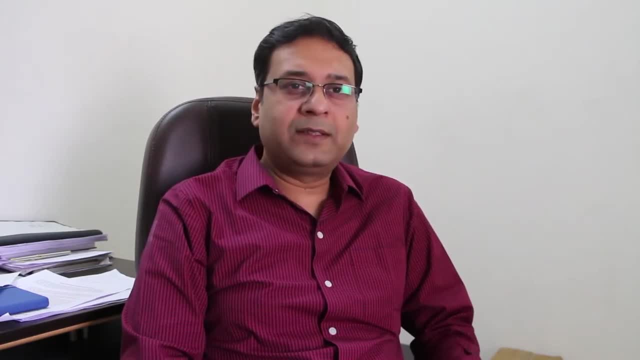 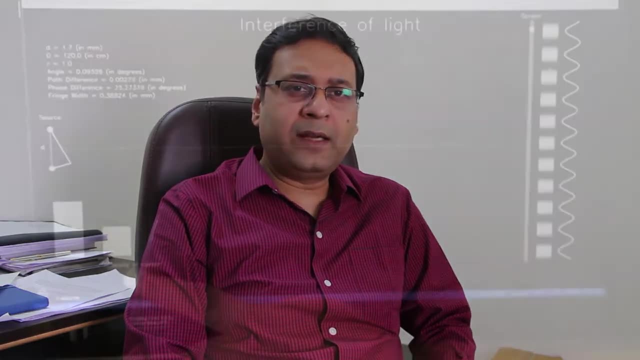 In undergraduate physics laboratory course, besides performing some classic physics experiments such as flanker experiment, diffraction, grating spectrometer, Fresnel bifrism, we encourage our students to get an idea of how real research is conducted. We ask them to form groups and come 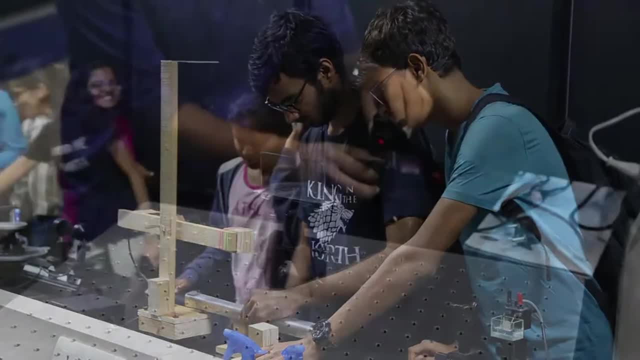 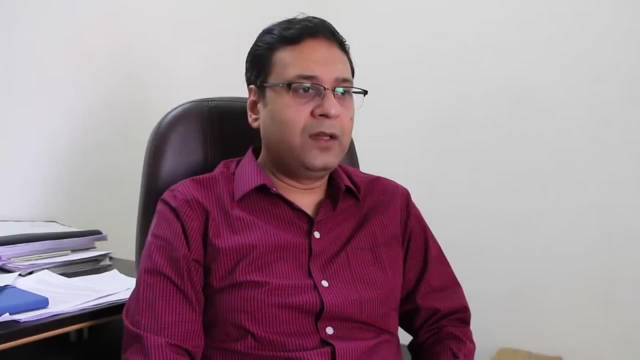 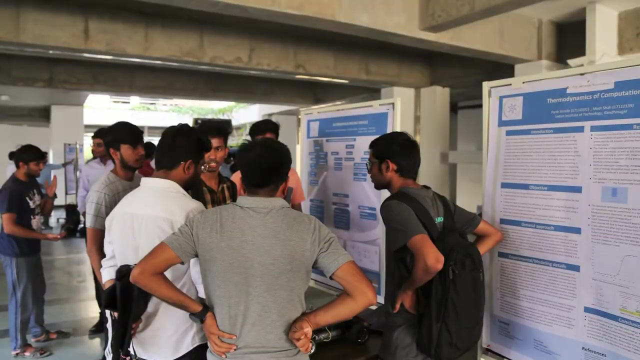 up with research proposals that eventually gets reviewed by the discipline faculty and, once approved, the students pursue those projects under the supervision of the same faculty. They are required to participate in a poster session at the end of the semester where faculty and students from other disciplines are invited to give their 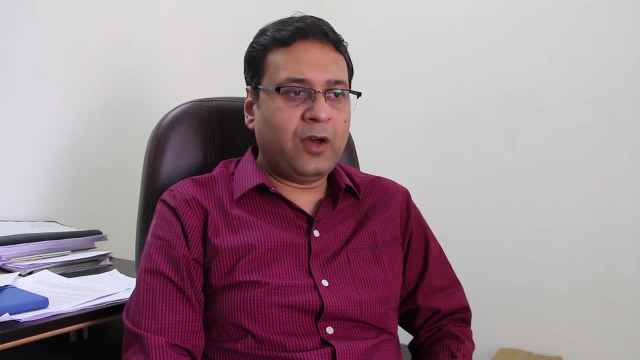 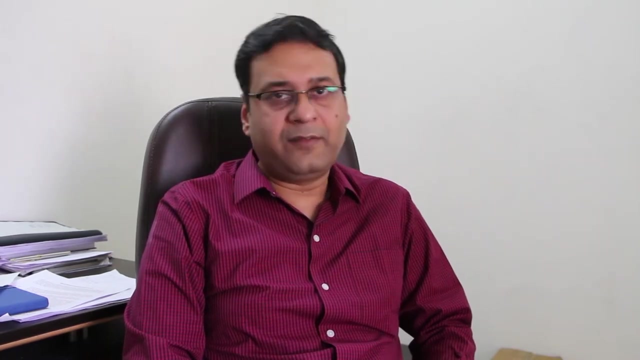 suggestions and feedback on the projects. We offer a very small amount of financial support from the discipline to each of these project groups, and the students are highly encouraged to reach out to other disciplines for help and collaboration and make the best use of the facilities that are available in the laboratory. 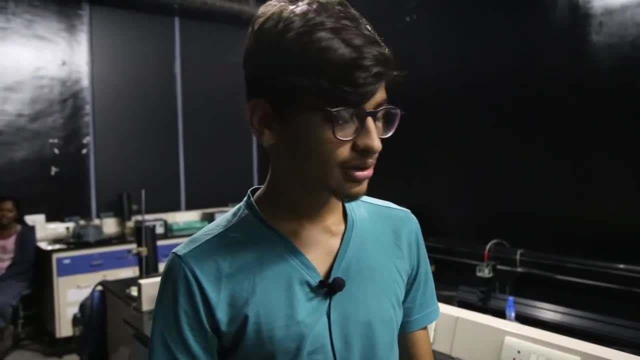 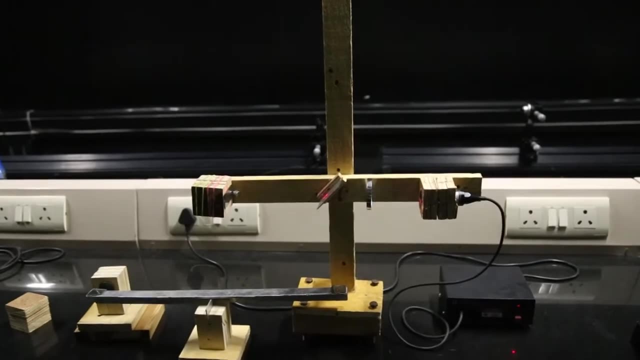 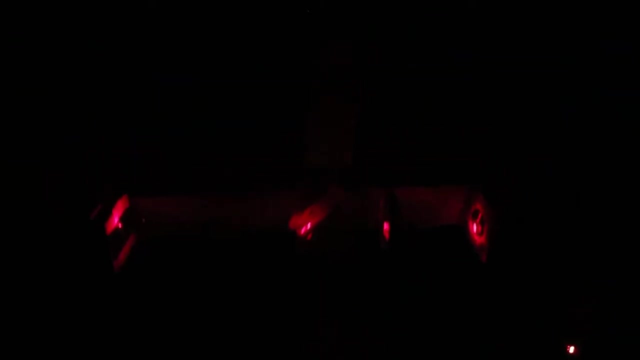 Hello. So the aim of our project is to measure the mass of microscopic objects using the principle of interference of light. So this is a setup which we made from scratch in the mechanical lab, and this is the laser, and the light then goes through the magnifying glass into the beam splitter, The 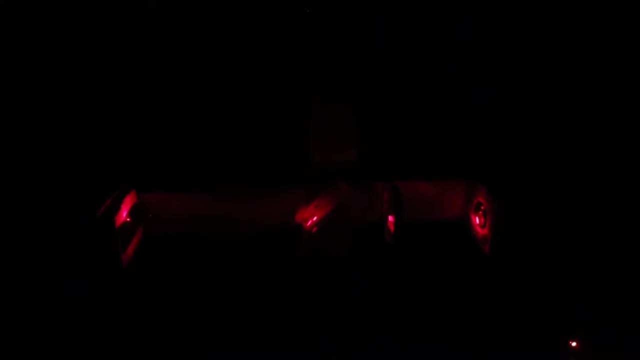 beam splitter splits the light into two beams. One beam goes into the mirror over here, as you can see, and the other beam goes down and both of them are reflected and in the end, going through the beam splitter, forms an interference pattern upon the screen. 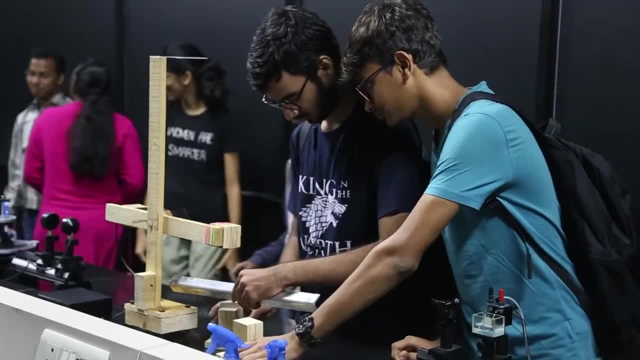 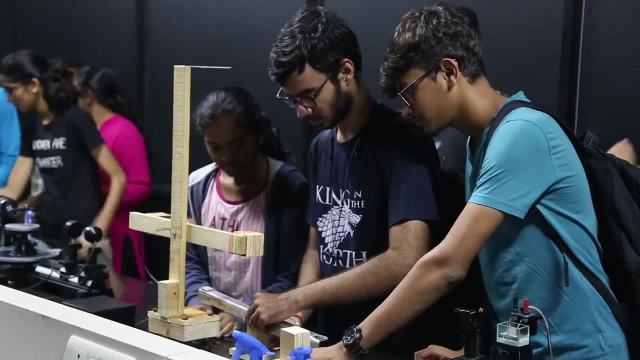 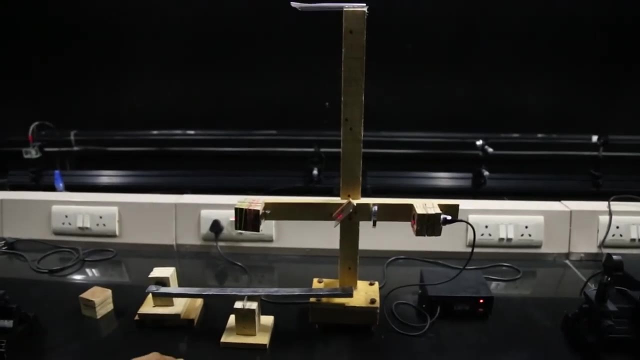 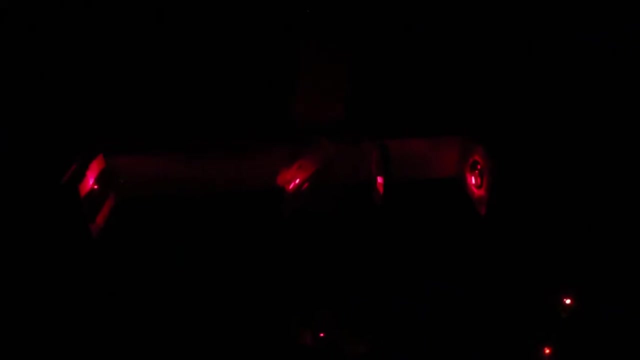 Here we are going to include this слишком small frame Going back to the element to show you how the beam will filed over that. Now, as one of the elements is teraz to that focal distance, the beam must be belong to there. linear, speechless gradient, that is. 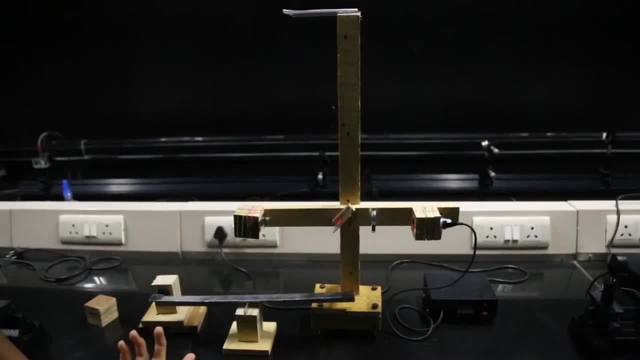 being replied as it is different. It means that the beam is not converging correctly And therefore the beam doesn't move as much in the�� it can rotate further and bigger distances within the circle using mass. Mosquitos use the concept of interference of light due to the path difference, the interference pattern. 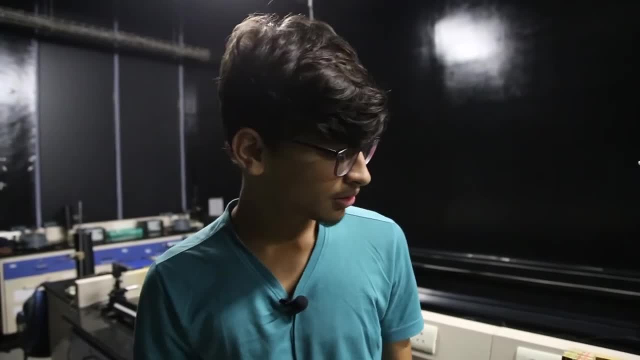 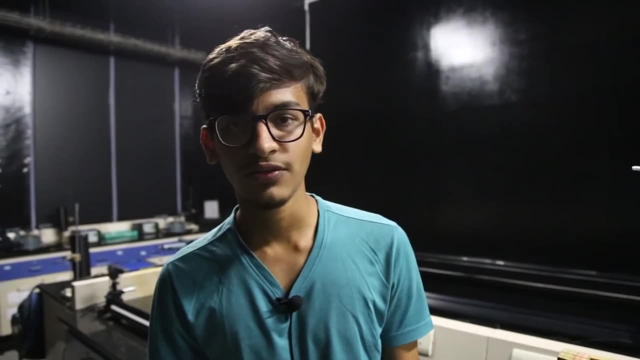 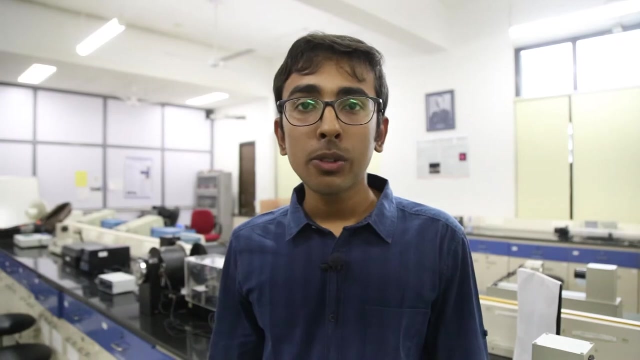 formed on the screen will change, and that will. that will be not be visible clearly, but we will use the principle of interference of light to calculate that and using a special formula we can calculate the mass of the object. our project is based on paper-based microfluidic chip, so